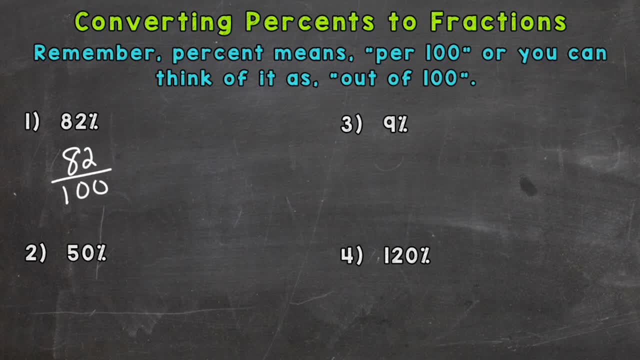 be 82 hundredths, or 82 over 100.. That's how you put a percent to a fraction. Now we can simplify that fraction, So a common factor between 82 and 100 would be 2.. It's actually the greatest common. 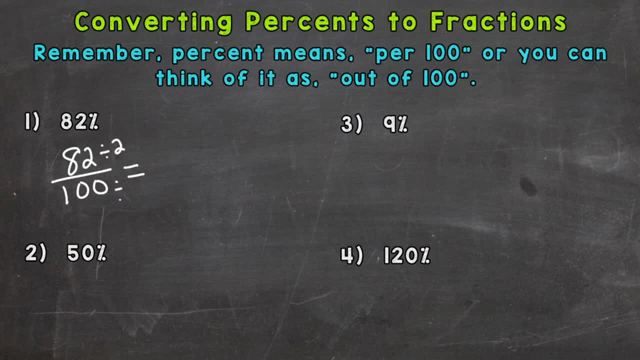 factor. So let's divide both by 2 to get our fraction in lowest terms. So 82 divided by 2 is 41, and 100 divided by 2 is 100. So that's how you convert a percent to a fraction. 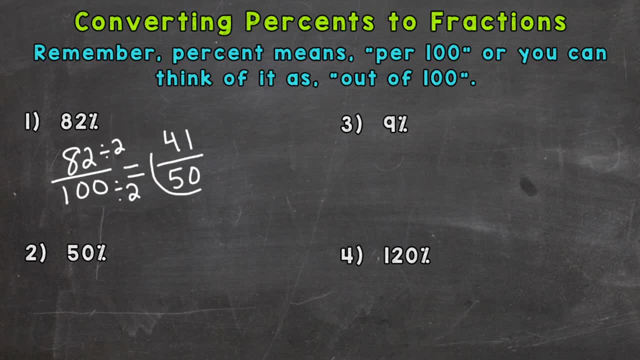 So again, percent means per 100.. So 82 percent means 82 over 100.. And then we simplify Number two: 50 percent, 50 out of 100.. And we can simplify this one: The greatest common factor between 50 and 100 is 50. We can divide both by 2.. So that's how you convert a percent to a. 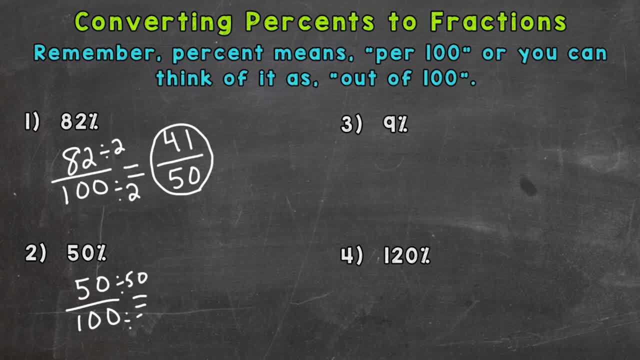 50.. And 50 over 100 equals a half, So 50 percent is one half. Number three: 9 percent, So that's 9 out of 100.. And that fraction is already in simplest form. So 9 percent equals 9 hundredths. 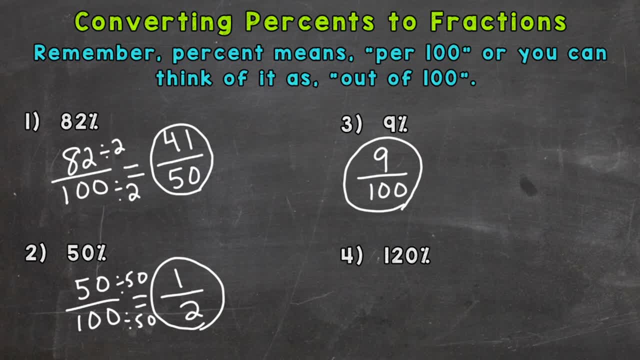 out of 100.. And number four: 120 percent. So that means 120 out of 100.. And that's an improper fraction, So it's going to be greater than one whole. We can pull one whole, 100 out of 120. 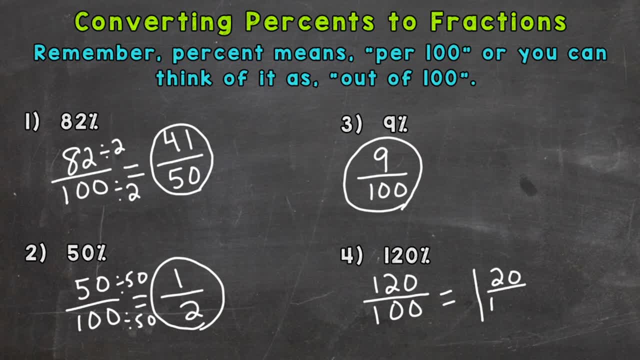 with 20 left over. Keep our denominator of 100 the same, And 1 and 20 hundredths can be simplified. The greatest common factor Between 20 and 100 is 20.. So we can divide both by 20. And we get 1 and 1 fifth. So there you have. 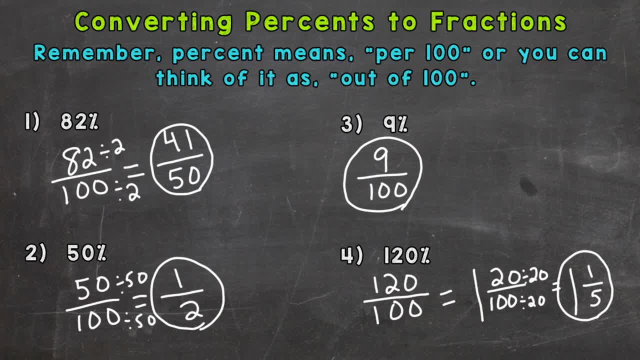 it. That's how we convert percents to fractions. We put that percent over 100.. It means per 100 or out of 100.. Hopefully that helped. Thanks so much for watching. Until next time, Peace, Peace.